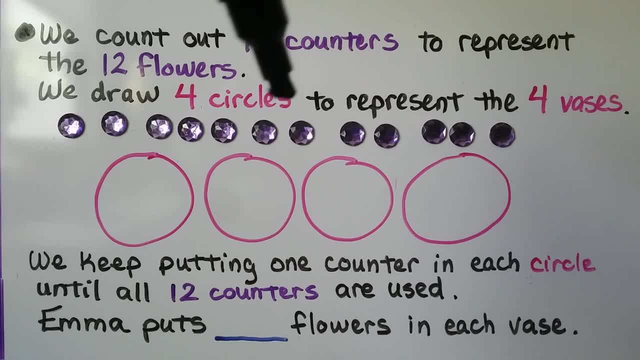 with three in each group. Here we have six counters, with three in each group. Here we have six counters, with three in each group. Here we have six counters with three in each group: four, five, six, seven, eight, nine, 10,, 11,, 12.. 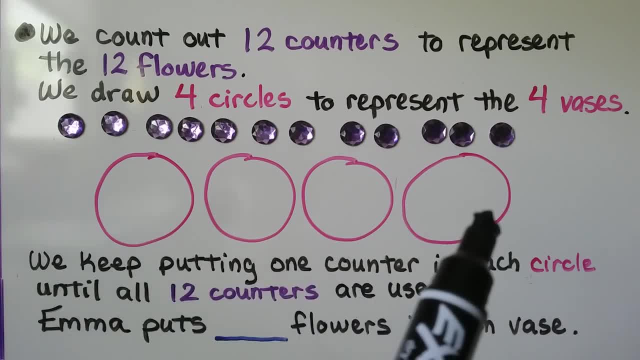 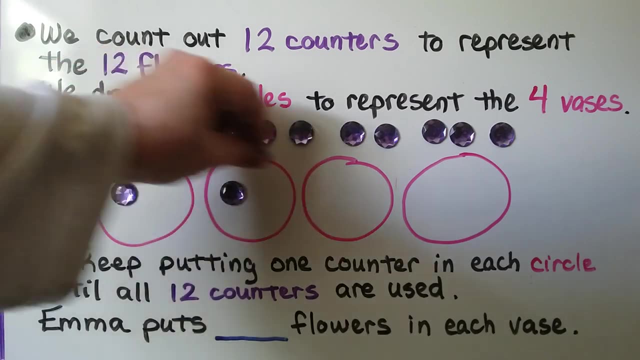 We draw four circles to represent the four vases And we keep putting one counter into each circle until all 12 counters are used. We take turns. we put one, then we put one in this one, we put one in this one, we put one in this one. 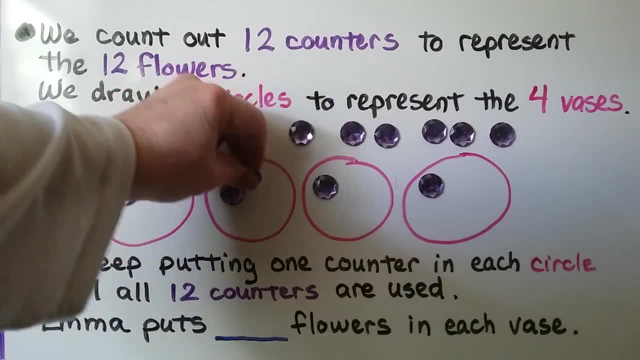 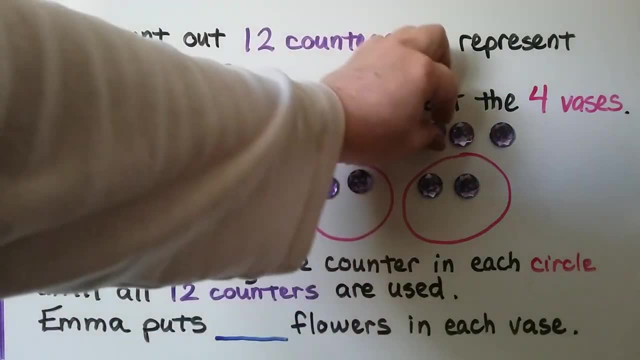 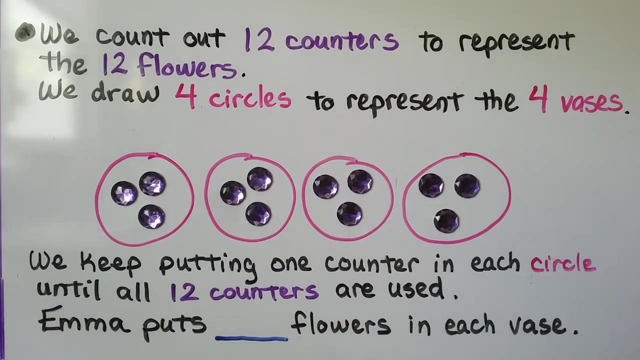 and then we go back and put another one in this one And we keep taking turns putting counters into the circles. Put another one here, put another one here and another one here, so that we have equal groups and all the counters are used. 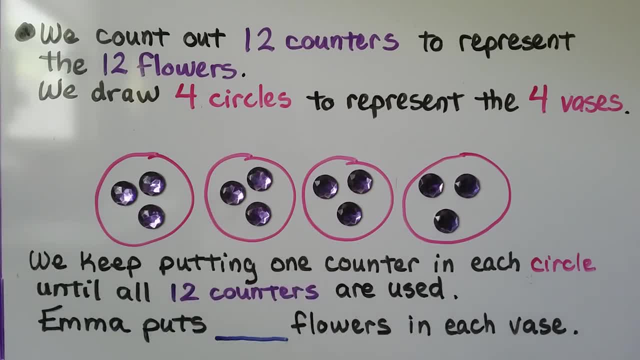 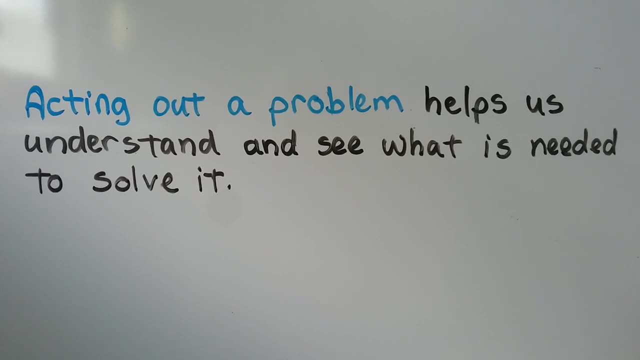 We can see there are three counters in each circle. That means Emma puts three flowers in each vase. Splitting up 12 counters into four groups, we have three in each group. Acting out a problem helps us understand and see what is needed to solve it. 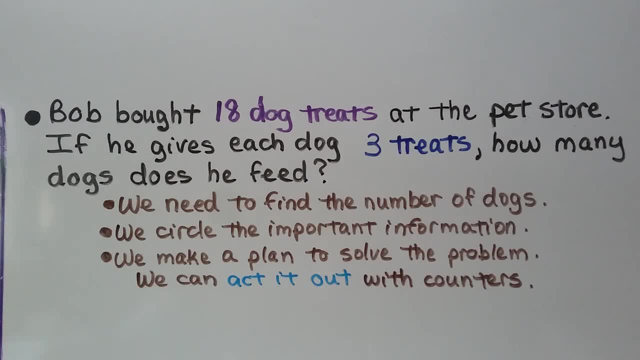 Bob bought 18 dog treats at the pet store. If he gives each dog three treats, how many dogs does he feed? We need to find the number of dogs. We need to circle the important information: He has 18 dog treats and each dog gets three treats. 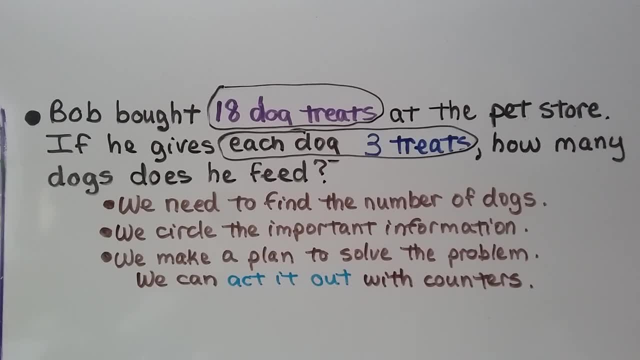 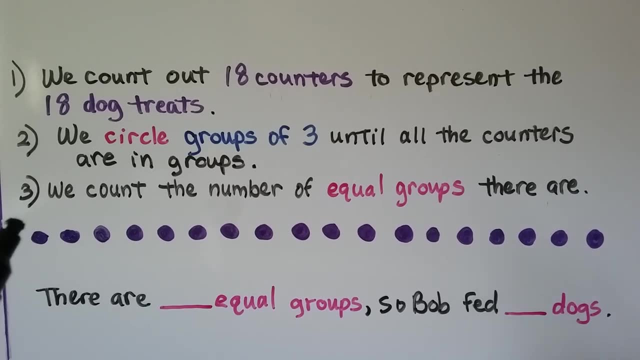 We make a plan to solve the problem. We can act it out with counters. We count out 18 counters to represent the 18 dog treats. We have one, two, three, four, five, six, seven, eight, nine, 10,, 11,, 12,, 13,, 14,, 15,, 16,, 17, 18.. 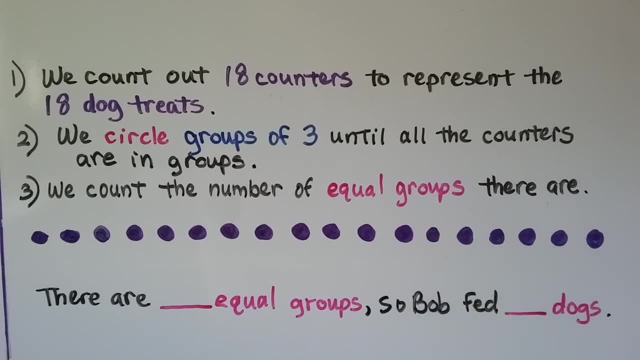 We circle groups of three until all the counters are in groups. That's one group of three, two, three, four, five, six equal groups of three. There are six equal groups. So Bob fed six dogs. We can imagine that each 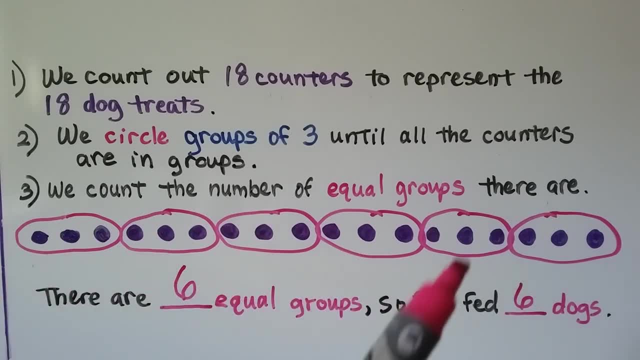 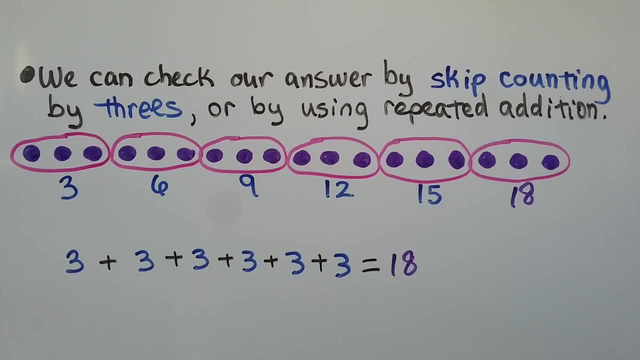 circle is a dog and there's six of them, They get three each. They're equal groups. We can check our answer by skip counting by threes or by using repeated addition: Three, six, nine, 12,, 15,, 18.. 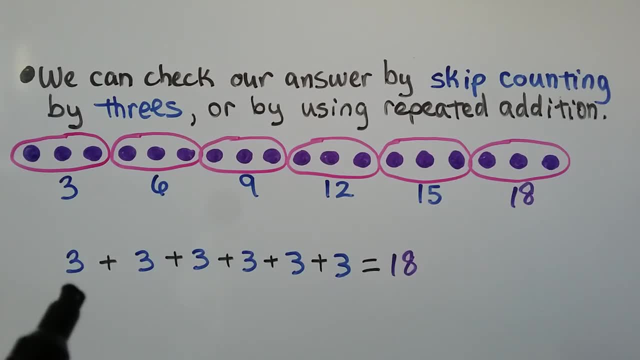 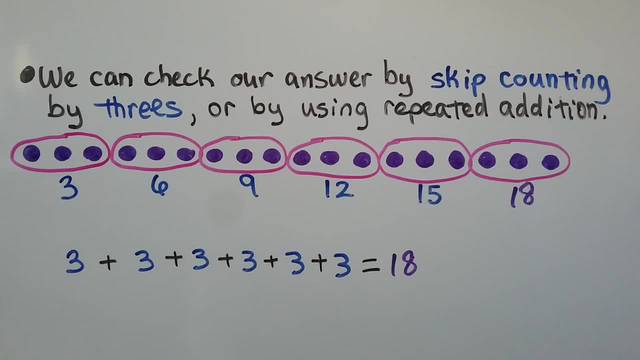 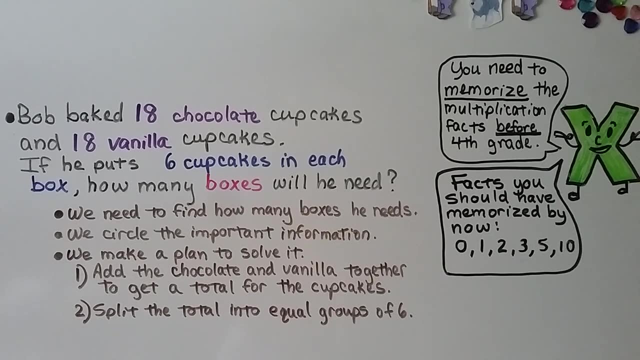 We add all these 3's and it's equal to 18.. So we know our answer is correct. Bob baked 18 chocolate cupcakes and 18 vanilla cupcakes. He puts 6 cupcakes in each box. How many boxes will he need? 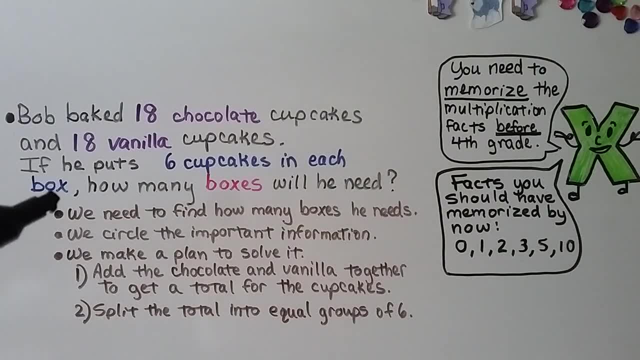 What do we need to find? We need to find how many boxes he needs for his cupcakes. We circle the important information: He has 18 chocolate, 18 vanilla and puts 6 in each box. We make a plan to solve it. 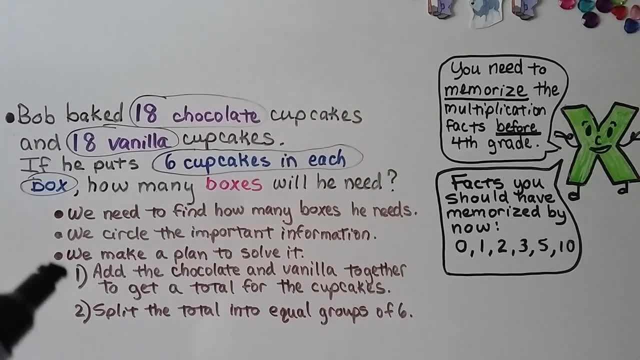 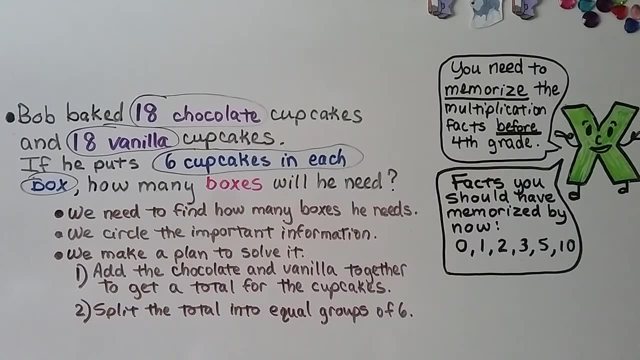 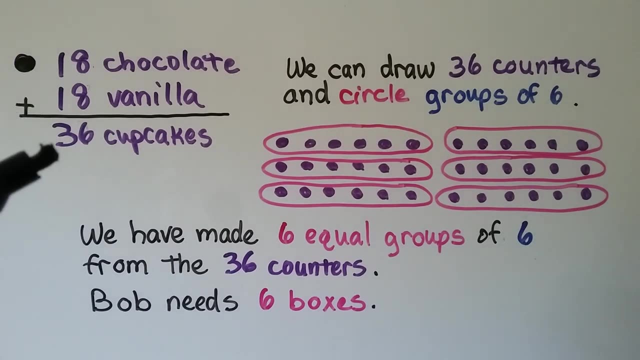 We add the chocolate and vanilla together to get a total for the cupcakes. Then we'll split the total into equal groups of 6. We can draw 3. We have 36 counters. 18 plus 18 is equal to 36 cupcakes all together. 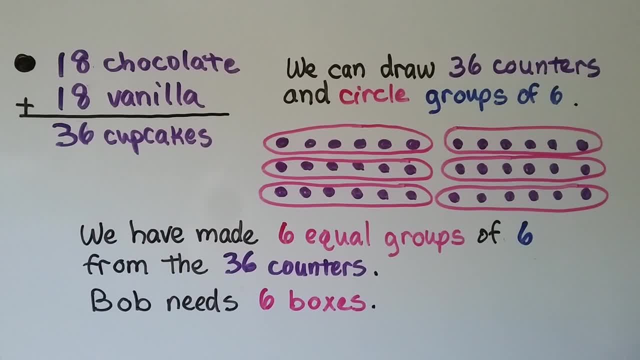 We circle equal groups of 6.. We have made 1,, 2,, 3,, 4,, 5, 6 equal groups of 6 from the 36 counters. That means Bob needs 6 boxes. We would have 6 boxes with 6 cupcakes in each box. 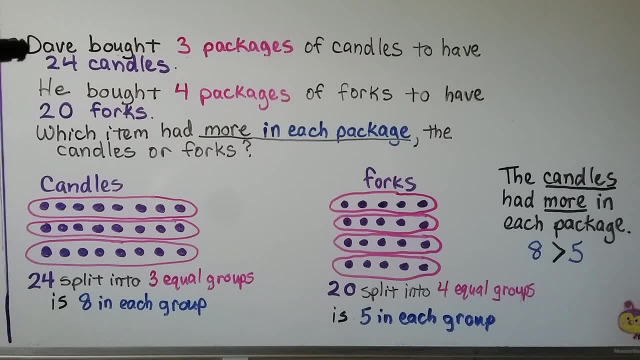 We then need to put all of the sense into this: 10 coins in together. Now we will split the total to get 3.. First we will add 4 into 16. When we have 2 more cupcakes to go, we add 4 as well. so we have 4 inserts. 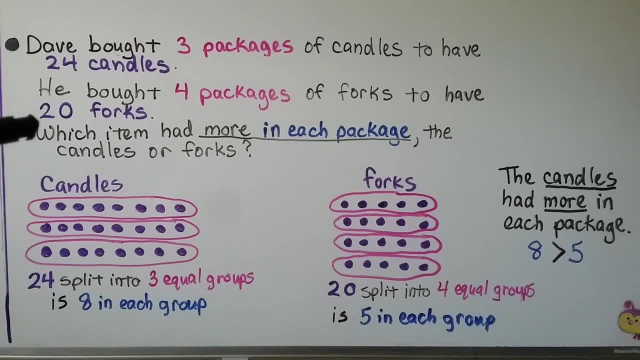 Then we need to put 1,, 2,, 4,, 5, 6 into this box. The first 24 are the stickers which comes in 3. We can consider all install 2 boxes by adding 2. Then we need to divide them in two. 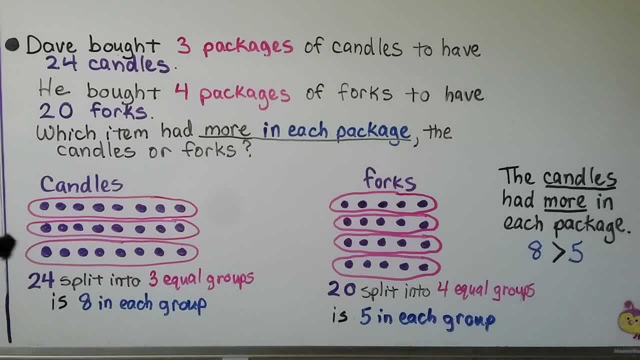 We single these out automatically by a number. ольш is a number of thirds. We bottom out this number And we add 2 to 8.. split into three equal groups is eight. in each group The four packages of forks that he has. 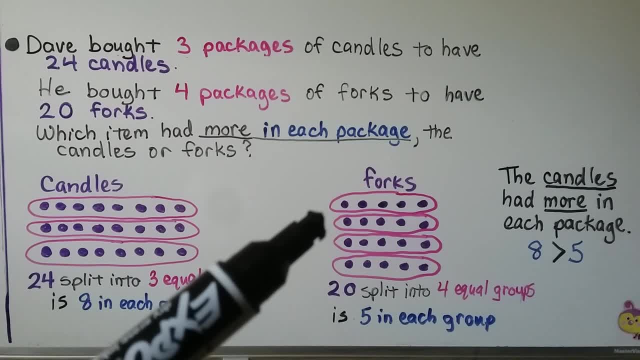 20 forks, we make 20 counters and we split it into four equal groups. 20 split into four equal groups is five in each group. Which item had more in each package? The candles or forks? We can see the candles have more in each group, don't they? The candles have more. 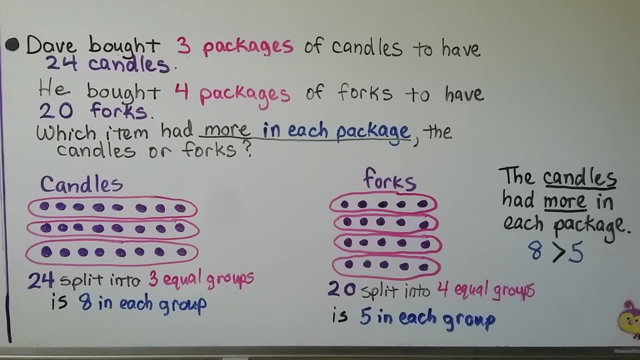 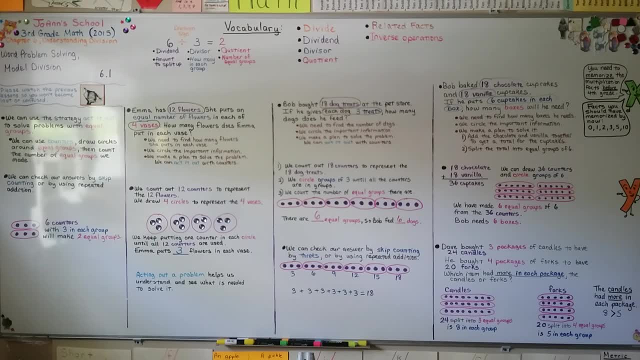 in each package. Eight is greater than five, So the answer is candles. So we can solve problems and model division by using counters or drawing dots for counters. You could even use bottle caps or pennies or some type of coin to be your counter. 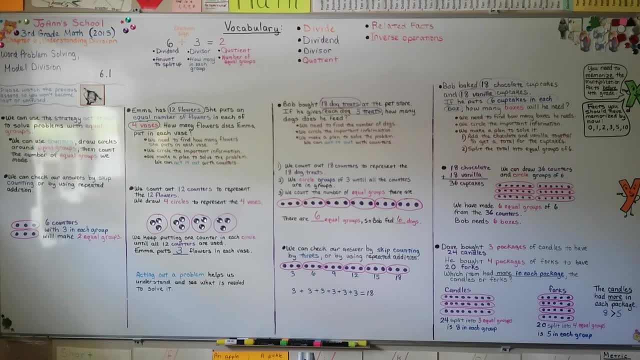 And you can put them into equal groups and find out how many equal groups you have. We're going to continue talking about division in our next lesson. I hope I'll see you there and I hope you have a really good day. Bye, Bye.